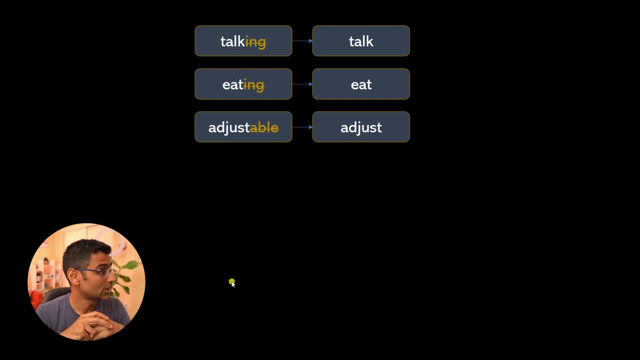 ing, you get the base word eating. there are other suffixes as well, such as adjustable. am I cable remarkable? so if you remove able, then you get the base word. So the point I want to make here is by using simple rules, without using any language knowledge, just by using simple rules, that. 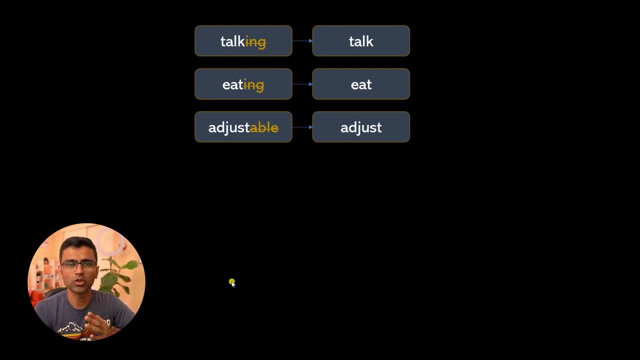 If the word has ing, remove ing or remove ing able. you can have a list of these suffixes and you can use the rule that remove these suffixes from a given word to get a base word. since we are using fixed rules or heuristic, this process is called stemming. 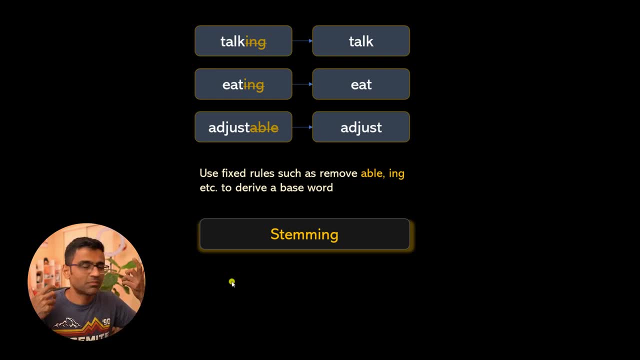 it's like stemming: you're just stemming the given word and getting the base word. but on some other occasions, applying just the fixed rule is not going to work. ate to eat. you can't apply this rule. you have to have that knowledge of that language. so whenever you want to use knowledge of the language or a 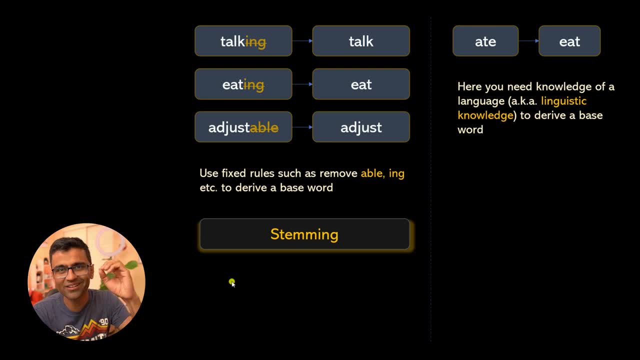 linguistic knowledge jargon alert. linguistic knowledge is nothing but a knowledge of a language. when you want to use that knowledge of a language and you get the base word, that base word, by the way, is also called lemma, so eat is a lemma for ate and this process is called lemmatization. 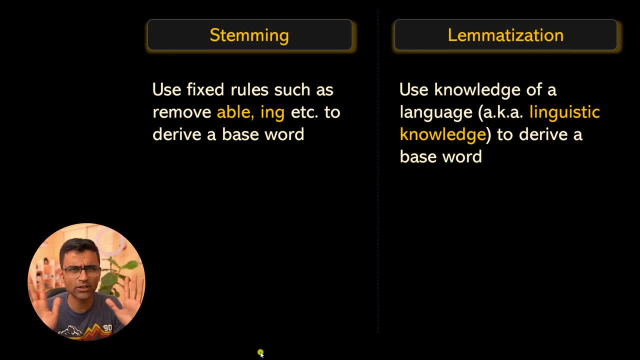 so stemming is just to summarize: using fixed set of rules, dumb rules- that remove this X number of prefixes or suffixes to get a base word, whereas lemmatization is little more sophisticated, where you need need to know the rules of that particular language. you need to have linguistic knowledge. 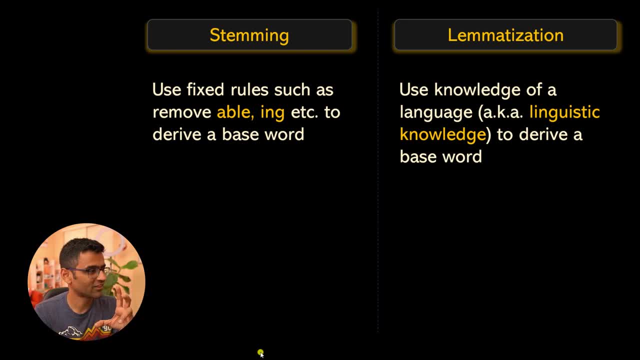 you might be guessing already that with stemming, you can get into issues sometimes. for example, if you have word ability, if you just apply the dumb rules, it will remove i ty and you will get this base word, a bill, which doesn't mean anything, where, as if you apply lemmatization, you will get the same word. 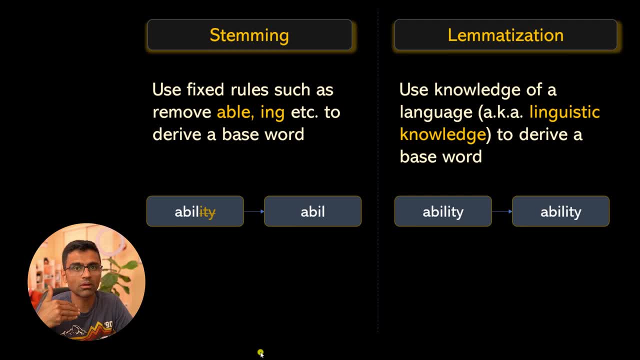 ability, but as you learn more about an LP application, you will realize that there is a value of based word ability. you will have babies level, but if you learn more about an LP application, you will realize that there is a value of both. so stemming and lemmatization, both are used and we are going to write some code. by the way, 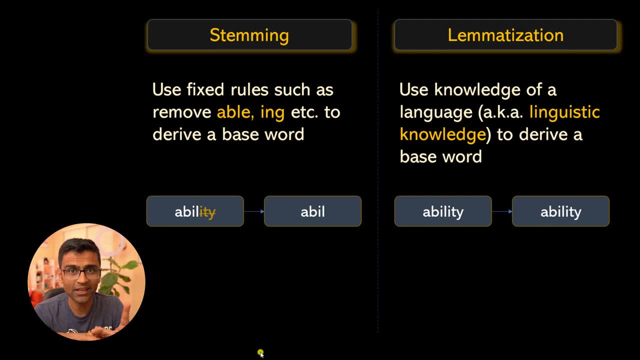 for stemming. we will use NLTK because spaCy doesn't have support for stemming. there is an article where spaCy authors have mentioned why they don't support stemming. because lemmatization, as you can already see, is more sophisticated, more correct, so they just have 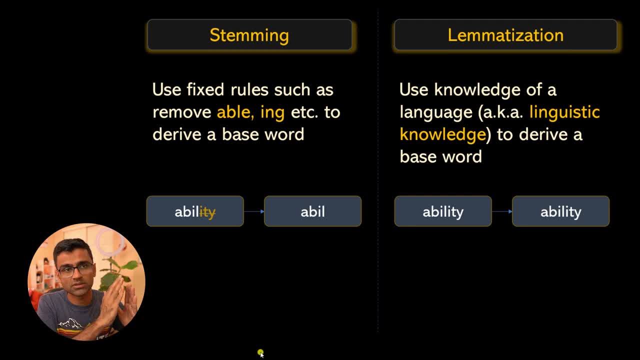 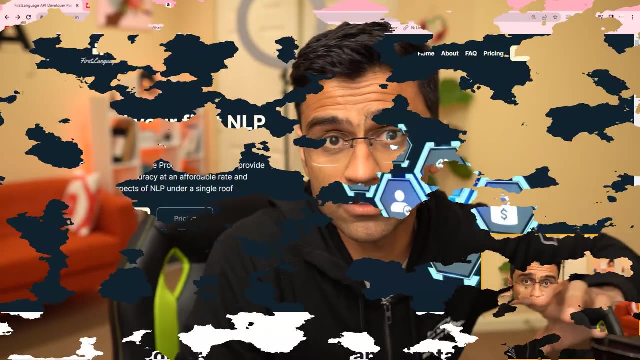 lemmatization support. but NLTK has both stemming and lemmatization- both they support both. so i'm going to show you NLTK and i will demonstrate stemming. i want to take a moment and talk about firstlanguagein, which makes building NLP applications easier for you. you can perform. 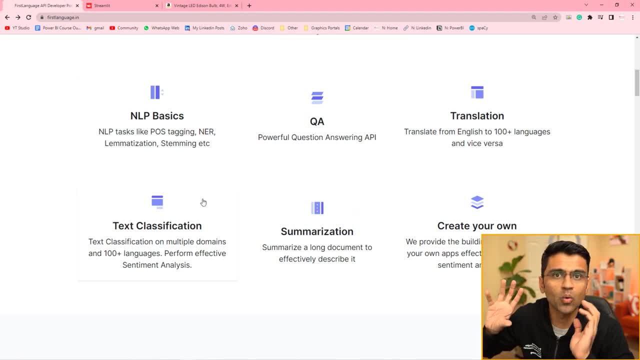 various NLP tasks which are shown here via this platform. if you're using a spaCy type of library, you can use this platform to build NLP applications. and you can use this platform to build NLP applications. you download it. you run your code locally. if you are training a heavy model, you need higher. 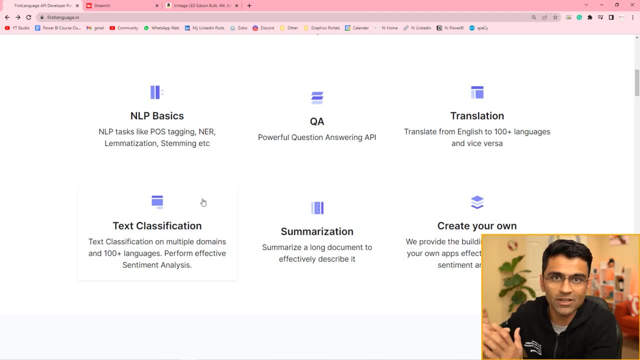 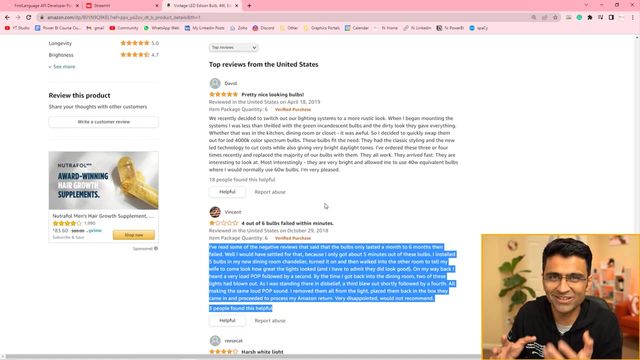 compute resources such as GPUs, whereas here everything is in cloud. you just make an HTTP call. things run on the cloud. you don't need a local machine with a lot of compute resources. there is a demo which you can see by clicking on this link, and i have bought this bulb recently. 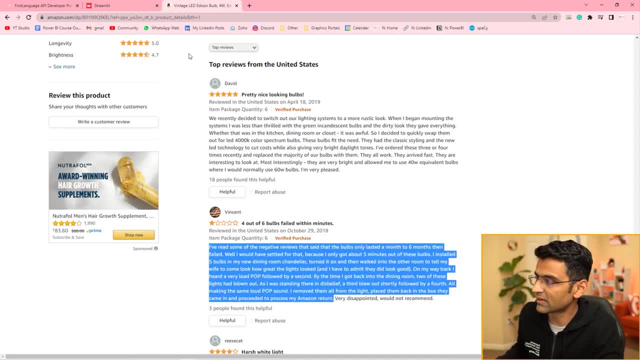 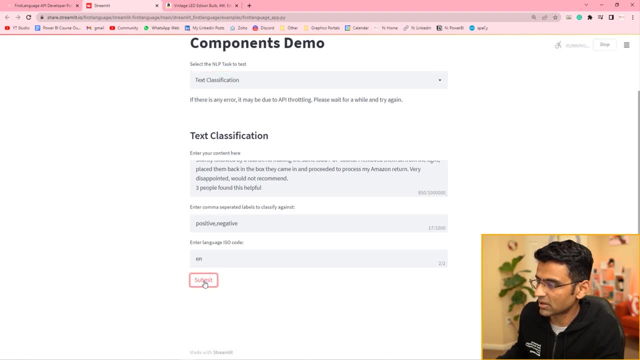 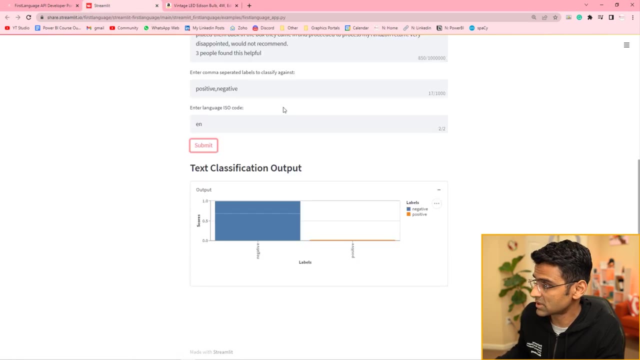 and you see there is a negative review on amazon and when i copy paste this here and i select text classification and when i say submit, it immediately classifies that as negative. and if i have a positive review, i just copy paste it here and if i submit it it will classify this. 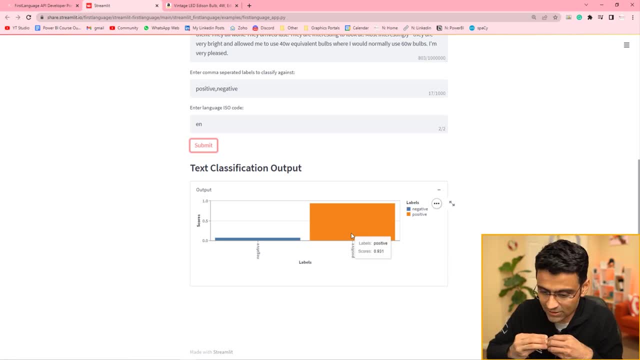 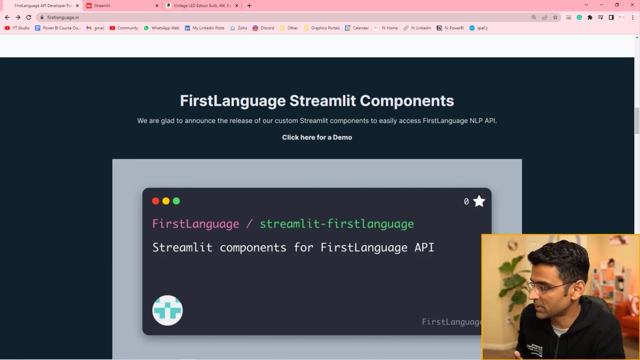 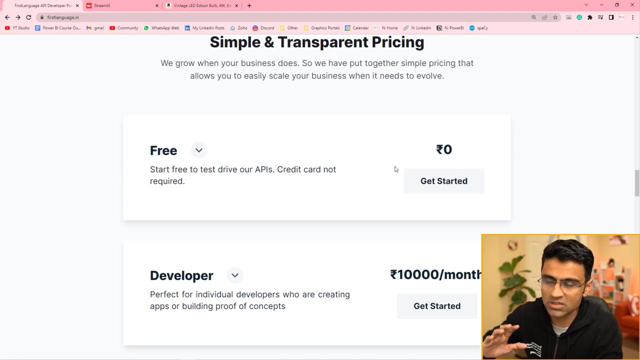 as a positive. see. it's pretty powerful, so it makes uh things much easier for you. you don't need to have like too much like detailed NLP knowledge. you can just call APIs and get things done quickly for yourself. the free tier is something you can try today. you can just sign in and you can get an API. 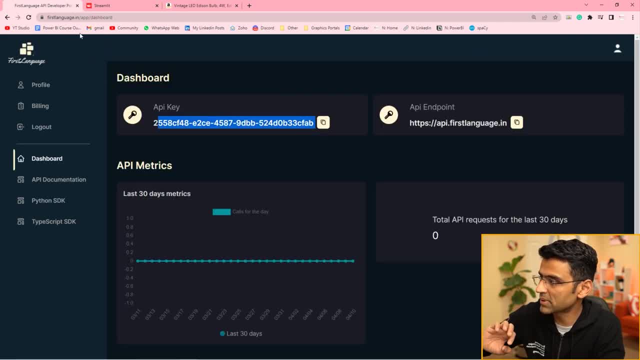 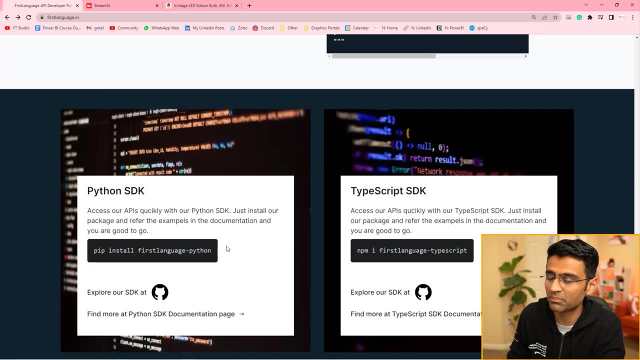 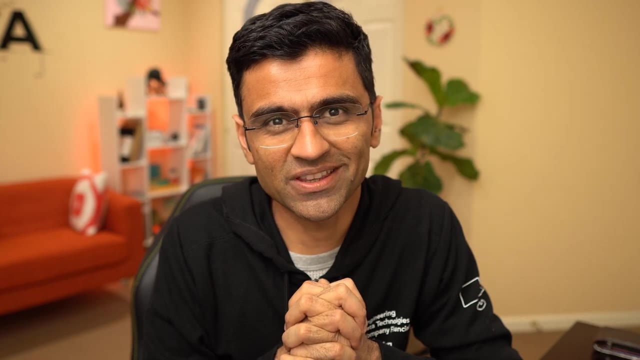 access once you sign in. if you go to dashboard, you will get your own API key and you can use that API key to make the calls. they have SDKs available both in python and typescript. go check it out. the link is in video description below. and thanks firstlanguagein for sponsoring this video. so let's 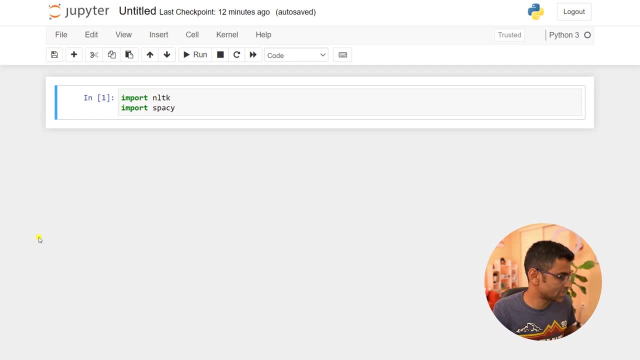 go to a notebook. so i imported. and, by the way, if you don't have NLTK install, you can in your command prompt. where is my command prompt? in your command prompt you can just run pip install NLTK- very basic right to install it. I have already imported both of these libraries and now I'm going to import Porter. 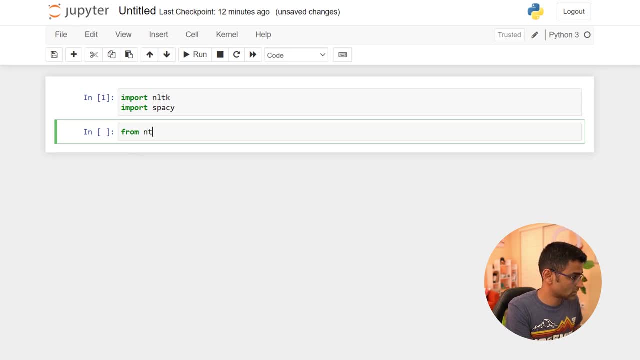 stammer from NLTK, so from NLTK, NLTK dot stem import Porter, you can just hit tab to autocomplete and stammer. this is a class, so I'm creating an object of this class in Python. when you do this, this is a class and you're creating an object of. 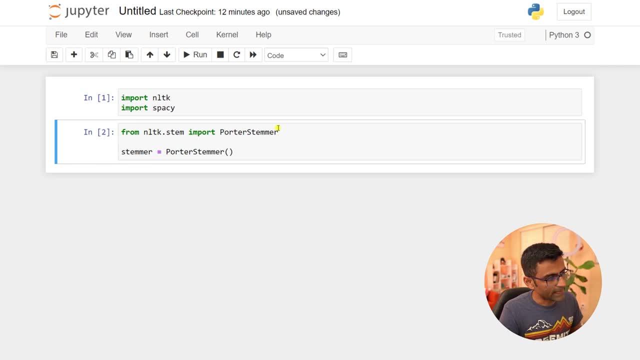 this class storing it here. that is other other other stammer as well, called snowball stammer. but I'm just going to show you one and I have a couple of words here and you can say for word in words print. so I'll print a word and then some separation, okay, and stammer dot stem that. 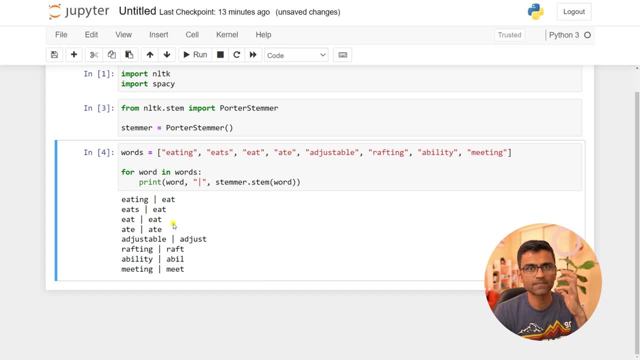 particular word and it prints the. thus it does the stamming and it prints the base word. so you see it applied fixed set of rules. so from it removed ing, got it. then when it has eats it will remove s and eat. if you have a base word, it will not do anything. 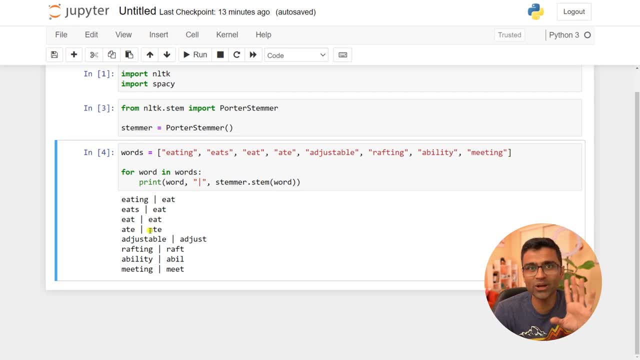 so eat, is it? but notice this ate. it did not do anything because stammer doesn't have a knowledge of a language. it is just using fixed rules, adjustable. it is saying: adjust rafting, raft and look at this ability. a bill. a bill doesn't mean anything, but still you will. 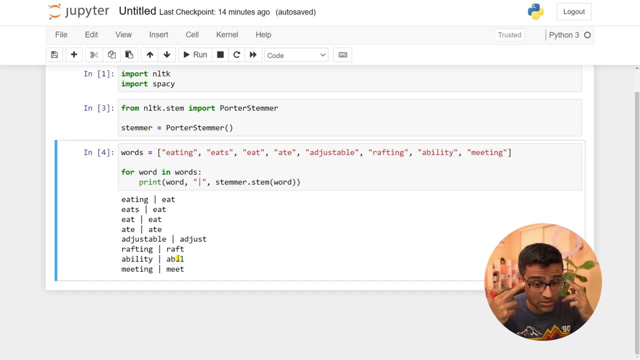 notice that many applications, even production applications, they use NLTK and using stammer could be efficient because it is faster, it just applies bunch of rules, it doesn't require any language knowledge and it can have a value in your NLP application. so although it is dumb, it can have a value. 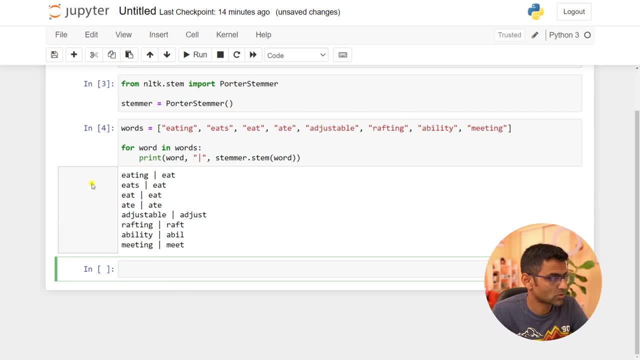 now let's do lemmatization in specie. so this was a quick demo of stemming in NLTK, so as usual. so I'm going to now create NLP object and say: specieload en core web. SM is small, you can use medium. I'm going. 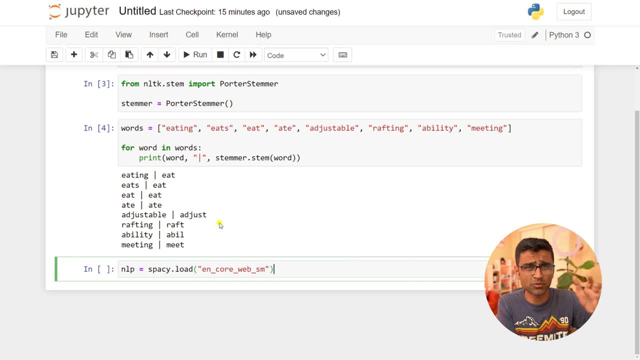 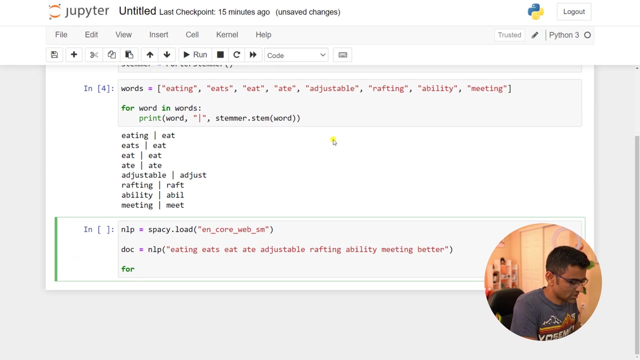 to use small version of English language processing pipeline. if you don't know what I'm talking about, you have to watch previous video and then I will create some document. so let's use the same word here. and since space is pretty straightforward, you can just say for word or for token in a doc. 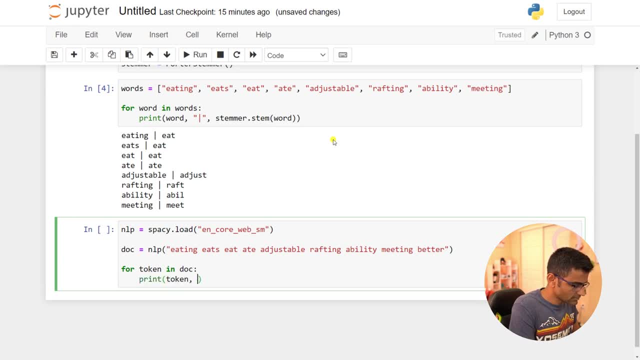 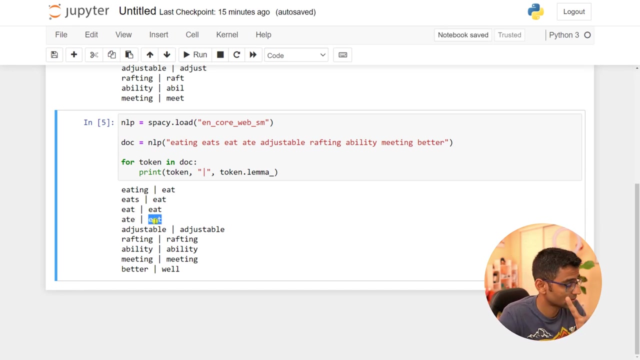 print, token, some separator and you can say: token dot, lemma underscore. notice this eight. it reduces to eat, eating, eat, see it worked fine. adjustable: it did not say just because the lemmatization, the rules which are set by default English model, says that the base word for adjustable 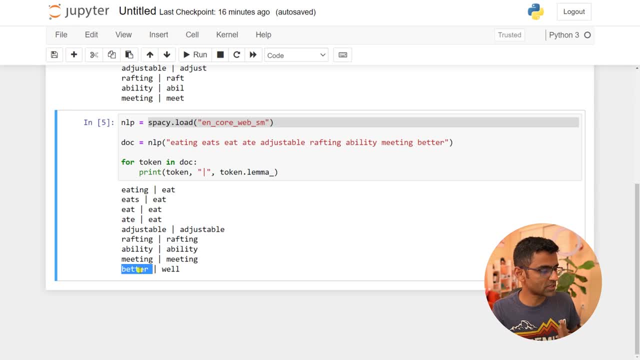 is adjustable. ability is the ability, but look at this when you have better. it reduced that word to well, so it has this mapping rules in the trained model that you just loaded. so, based on the language, based on what kind of model you're loading, you might be loading a different. 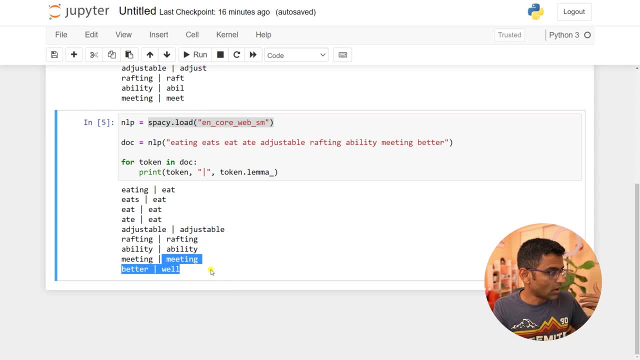 English model, which will have a different rule. so there is. this is a quick demo of lemmatization in specie, if you. by the way, let me show you one more thing. let's see which is this, this thing called token dot lemma. so see, there is lemma. 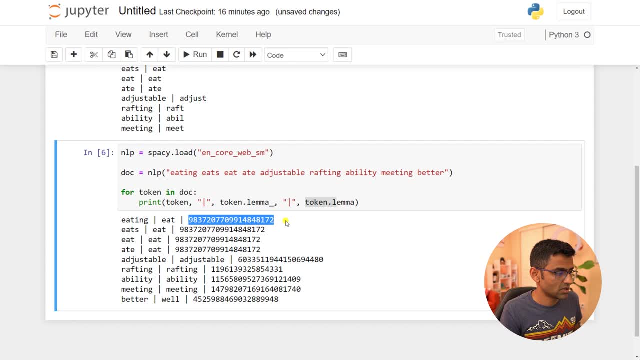 and there is lemma underscore, so lemma is just printing a hash. so it's a unique hash of your lemma, which is a base word because this is a train English model with a fixed vocabulary. it has few thousand words and for each word it will have a unique identifier, short of and. 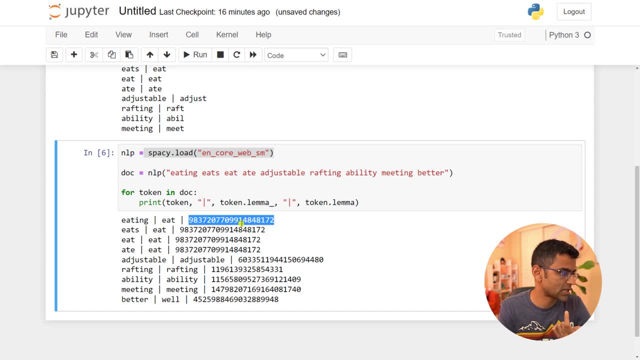 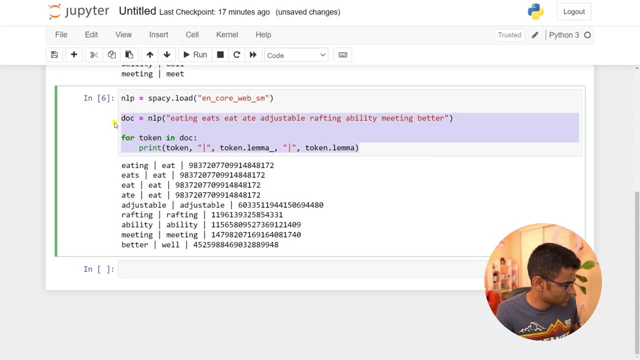 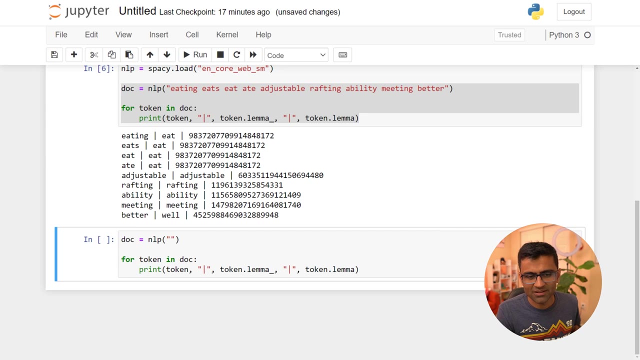 that is this hash, and you'll see that for eat, the hash is same. this is just for your knowledge. by the way, I just wanted to quickly show you different sentence, so I'll just do copy-paste and I will try. I don't know if you all watch Mandalorian, Mandalorian. 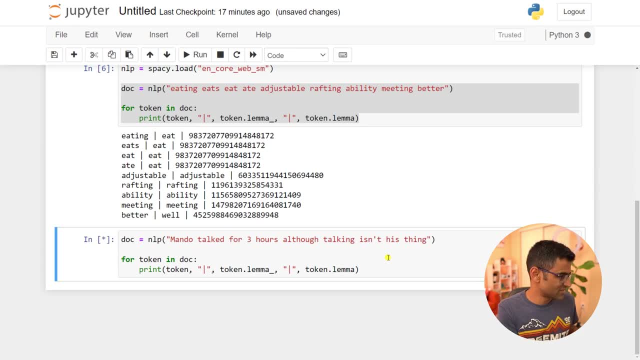 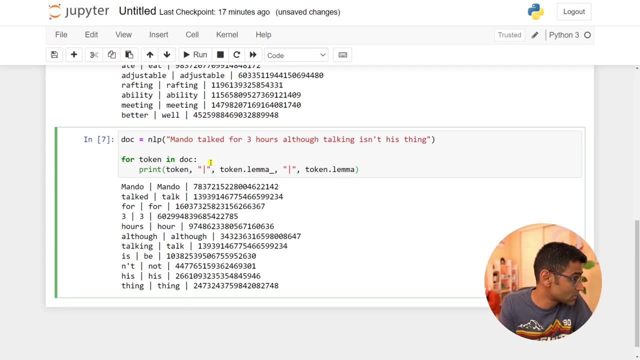 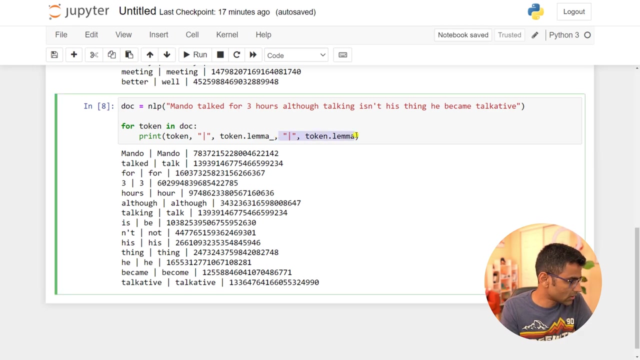 is my favorite series on Disney, so Mando doesn't talk that much, but Mando talked for three hours. hooray, Mando is becoming talkative. Mando talk for three hours, although talking isn't his thing I, he became talkative, so sit top. it reduces to talk, talking is. 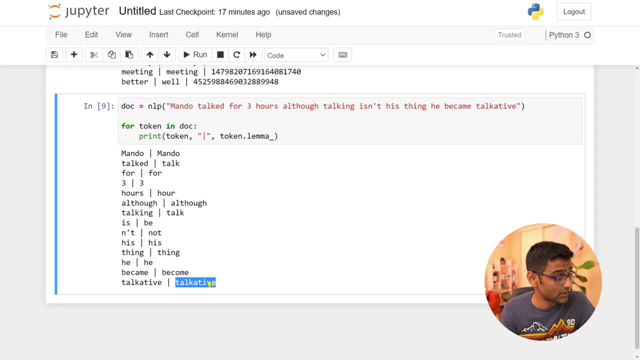 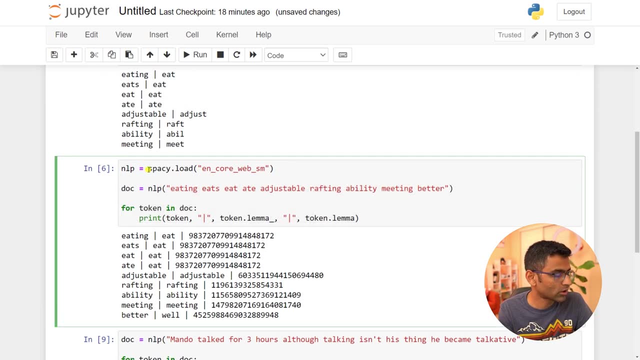 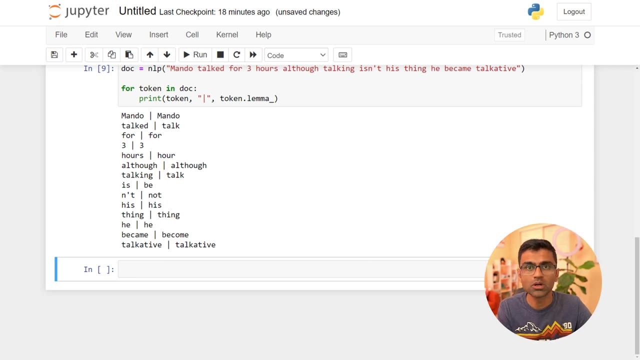 also reduced to talk, but talkative is still talkative, because this is, this is how, as I said, this is how this particular model behaves. sometimes you might want to modify a behavior. right, you want to customize it, so how do you do that? so, if you remember our pipe names, so we have. 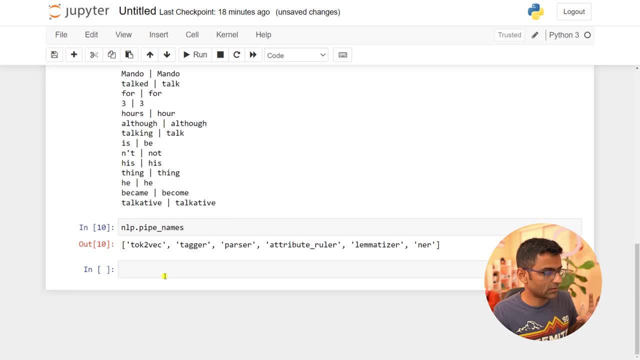 for this particular model, the pipeline that we have is this: there's a talk to actor, tagger, parser, attribute ruler and then there is a lemmatizer. now attribute ruler assigns attribute to a particular token and you can customize it. so let me explain what what I mean here. so let's say you have 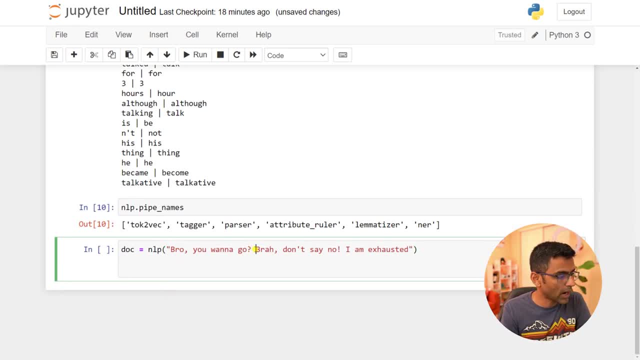 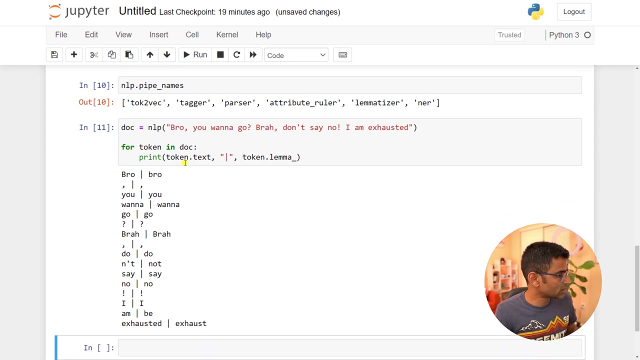 this sentence now: bro bra brew, all these are the. you know you mean brother basically, when you say this, but by default the language model doesn't understand. this is slang, right? so it doesn't understand. so it will say: bro is bro, bra is bra, right. and if you look at the first token itself, so 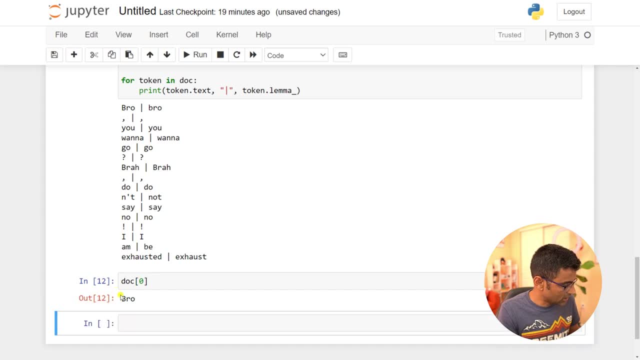 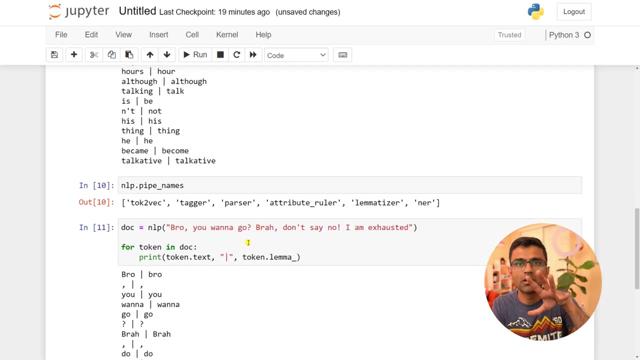 like the first token. is this correct bro? and if you look at the lemma of that, it is bro, because it doesn't understand the slang. but let's say you want to customize this model. you know that bro and bra means brother. you can customize it by doing this. so what you do is you. 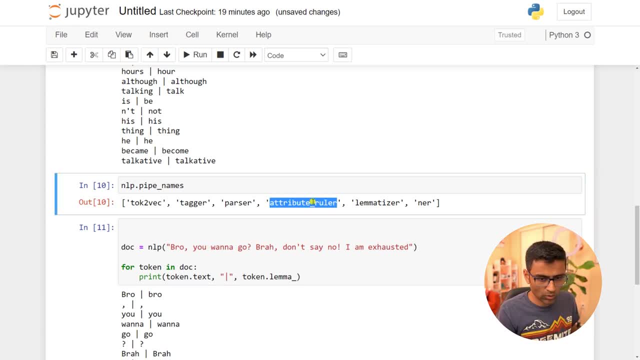 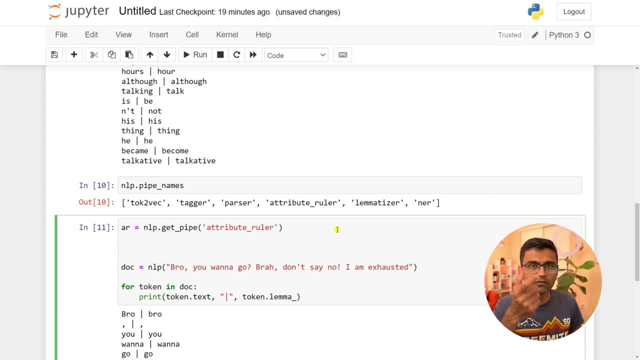 go here you get this particular attribute ruler by doing this. so you'll say nlpget pipe attribute ruler, so it will give you that particular component from the pipeline and then you can customize it by adding that custom rule. okay, so see, here I am adding a. 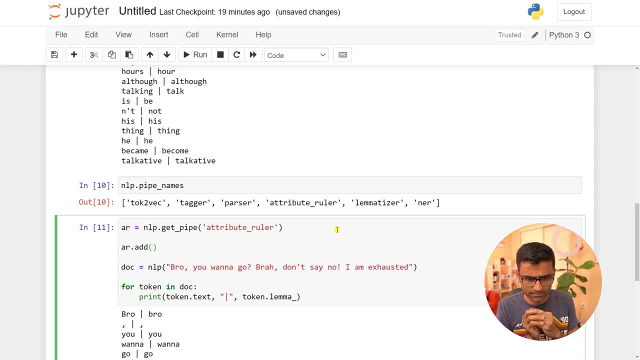 custom rule where I am saying this. so what I want to say is: I want lemma to be brother. so for bro and bra, I want their lemma to be brother. okay, so here you are assigning attribute and attribute is lemma. so basically you're saying the lemma for. 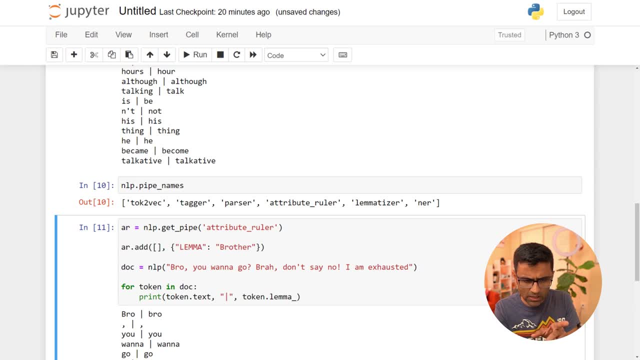 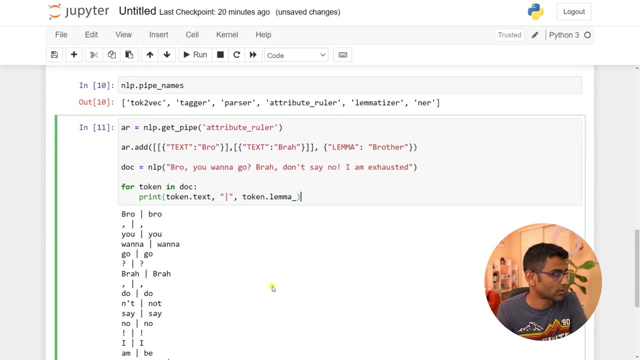 the words that I'm going to specify here and the way you specify those words. I mean, that is this, I'm just going to copy paste. you're saying for brother, bro and bra make their base word to be brother. so you notice, previously bro was bro and 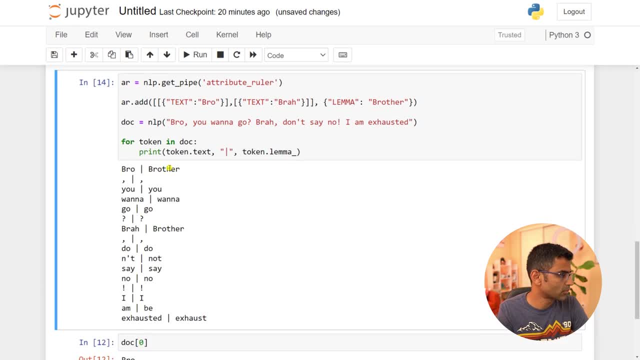 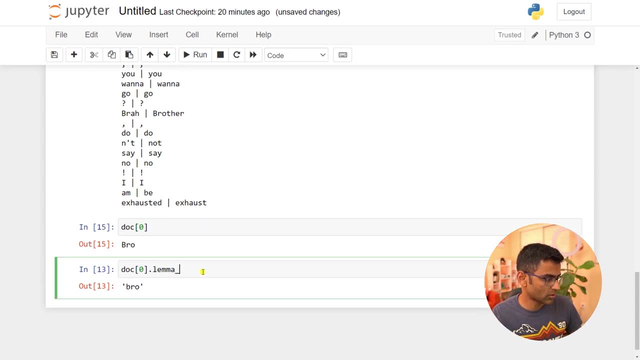 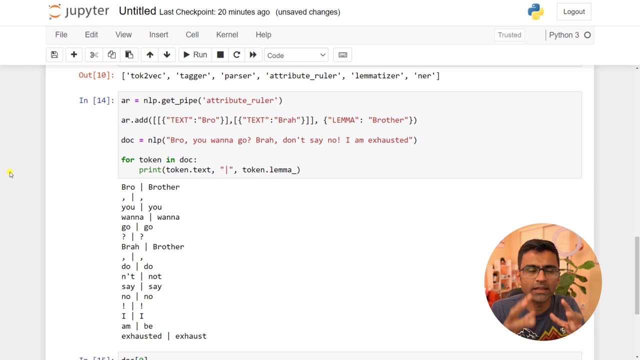 bra was bra, but when I run this again, bro is brother and bra is also brother and for the bro see the lemma was bro but now the lemma became brother. so I hope this gave you a some understanding of stemming and lemmatization. I don't have an exercise. 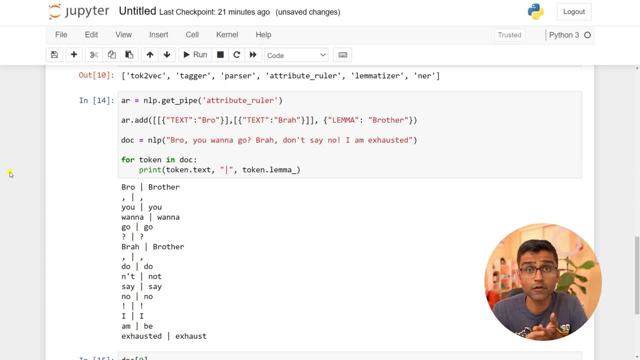 for this particular video, but i might add exercises in the future as well. so always check the video description below, because sometimes, if i don't find time for the exercise while recording this video and if i find time later on, i add those exercises and i i talk about.